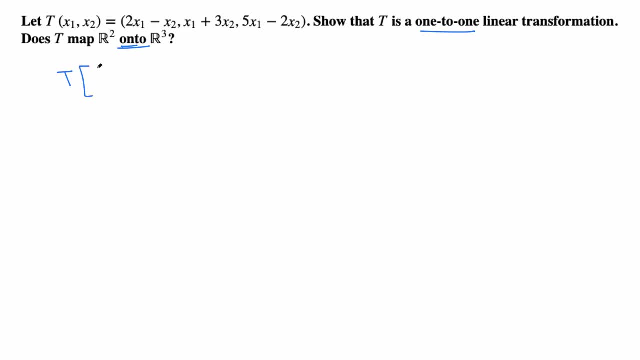 transformation. so T of x1, x2. you can write in this way in vector notation in vertical. so this is the case- is 2x1 minus x2, x1 plus 3x2, 5x1 minus 2x2, and this vector is in fact. we can write in this way. so we got x1- x2. 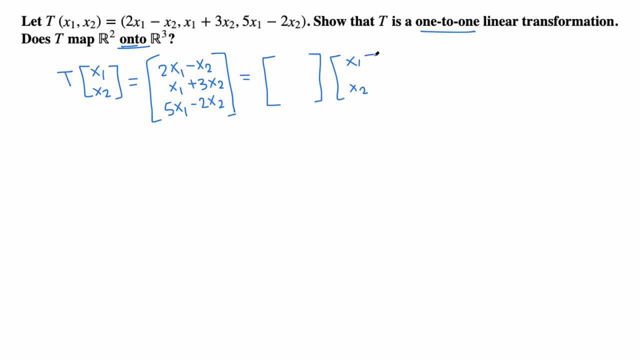 that goes here and just the coefficient now: 2, negative 1, 1, 3, 5, negative 2.. Okay, so this transformation is in fact given by t of x, because vector x, t of x, equals ax. Since it's given in this way, we can write in this way: t of x equals a of x. 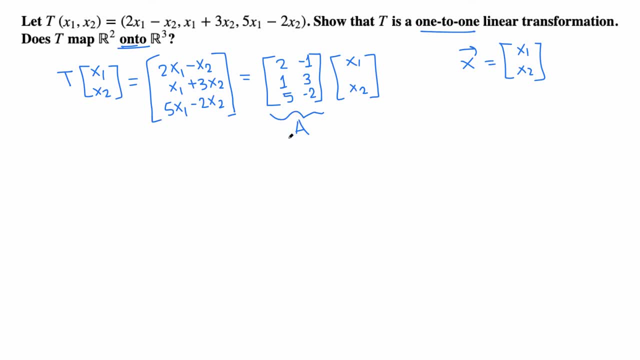 where a is the standard matrix. so this is indeed a linear transformation. okay, Linear transformation, because we can represent this by this standard matrix. Now we need to show: t is one to one linear transformation. So look at the columns of these two, of this matrix. 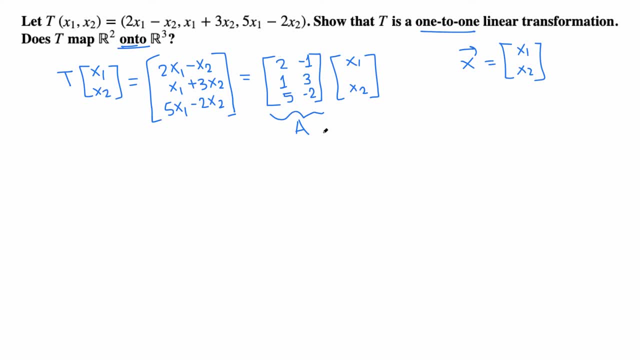 These columns are linearly independent because whenever we have only two vectors, if one is not constant multiple of the other, then they are linearly independent. So t is a linear transformation. with the standard matrix a, or since we got a matrix a, this is a linear transformation. 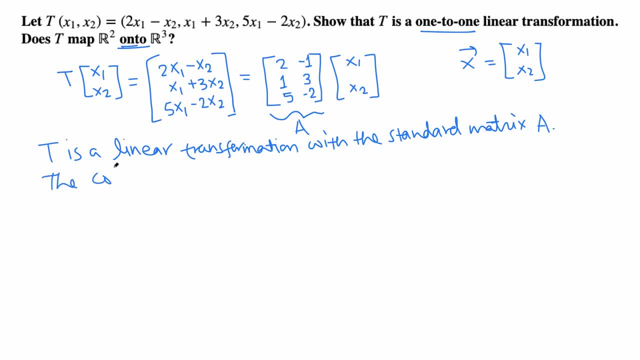 and the columns of a. the columns of a are linearly independent. I'm writing a linearly independent. One column is not a multiple of the other. Okay, since the columns of a are linearly independent, let me put: since the transformation t is a one-to-one. 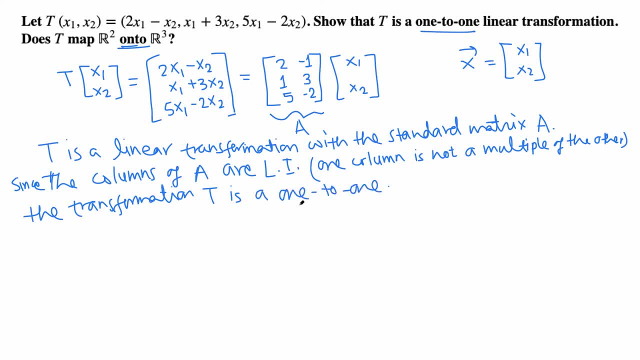 linear transformation. So because this matrix got two columns and these two vectors or these two columns are linearly independent. Now next we want to see if t also t maps R2 onto R3. So for this one, so onto R3 means for any vector in R3, any. 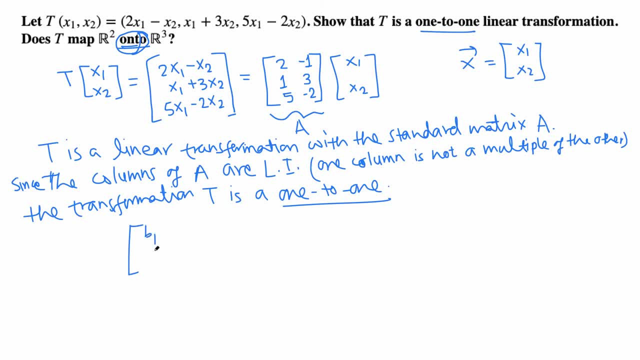 r3 any vector means we have, let's say, b1, b2, b3, a generic vector, that's in r3.. Can we find x1, x2? okay, for any vector. can we find x1, x2 in r2 for any vector? can we find x1, x2? 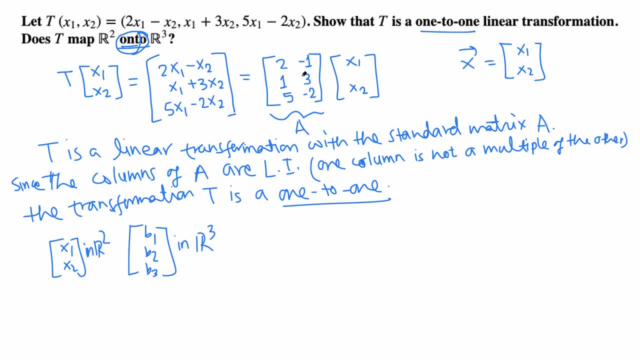 so that when we map in this way, when we multiply this by a, we get this vector. is that possible? It's no, because there are only two columns or only two vectors to generate a vector like this. okay, we don't need this to generate a vector in r3, we need three columns, three linearly. 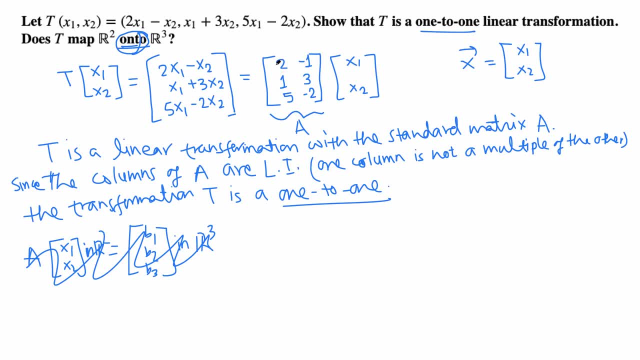 independent columns, by the way, or we need three pivot positions, okay, in the row, so so we can have one maybe here too, but we have only two columns, so there is no way we can get three pivots rows. okay, this is going to be 0: 0..